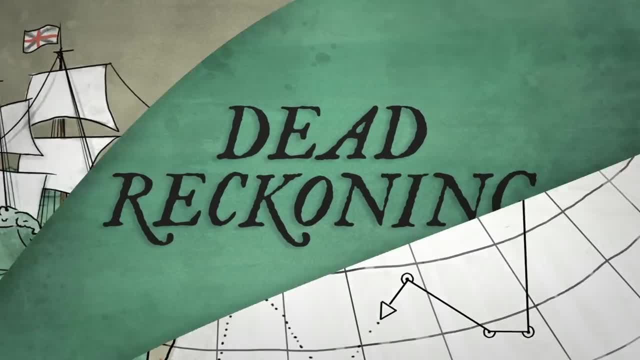 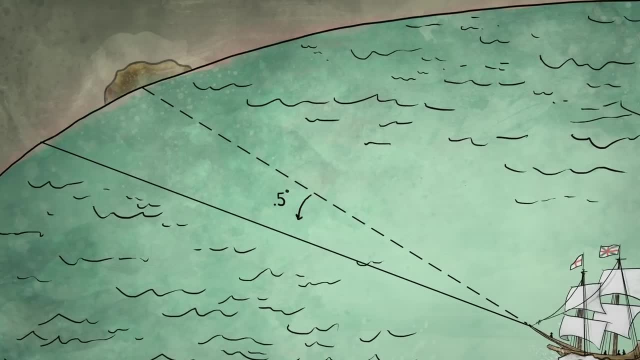 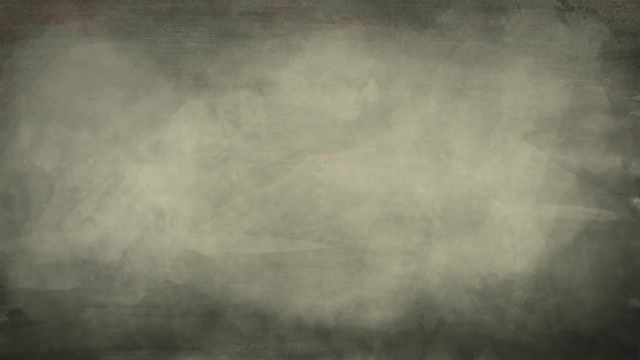 and the distance sailed. This process was known as dead reckoning, because being just half a degree off could result in sailing right past the island that lay several miles just over the horizon. This was an easy mistake to make. Thankfully, three inventions made modern. 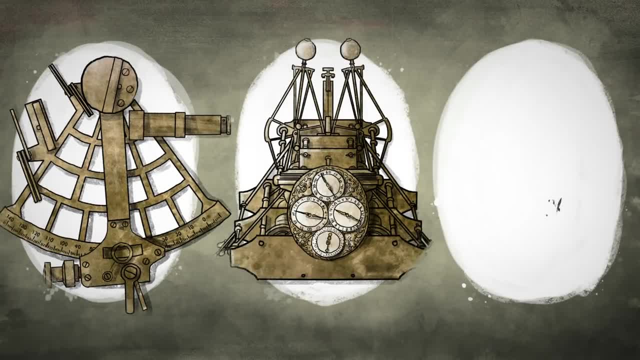 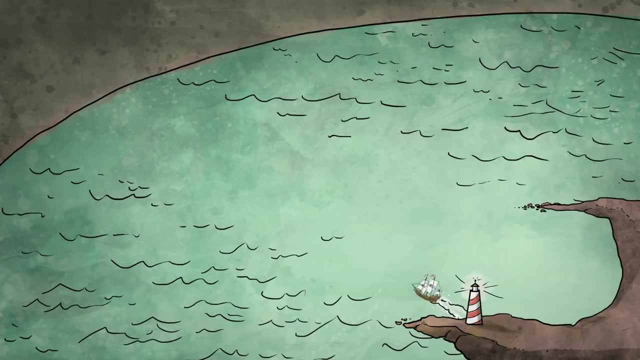 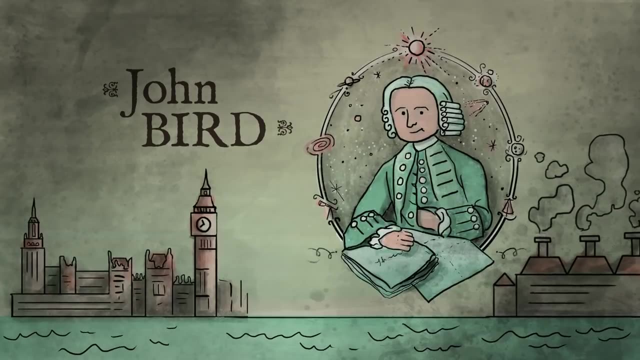 navigation, possible Sextants, clocks and the mathematics necessary to perform the required calculations quickly and easily. All are important. Without the right tools, many sailors would be reluctant to sail too far from the site of land. John Byrd, an instrument maker in London, made the first device that could measure the angle between the 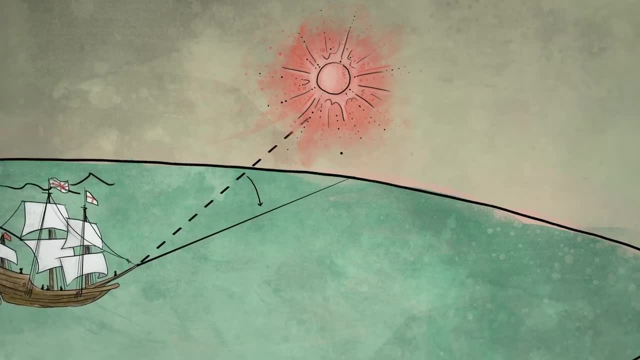 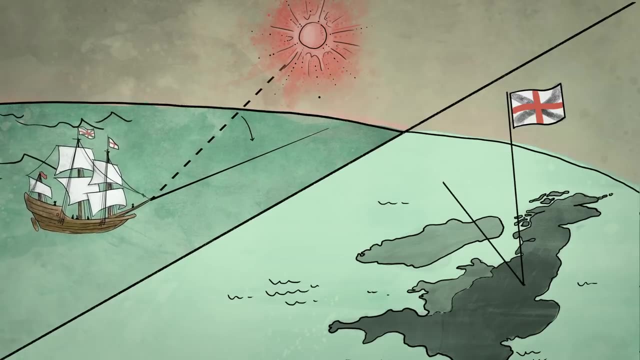 sun and the horizon during the day called a sextant. Knowing this angle was important because it could be compared to the angle back in England at the exact same time. Comparing these two angles was necessary to determine the longitude of the ship. Clocks came next In 1761,. 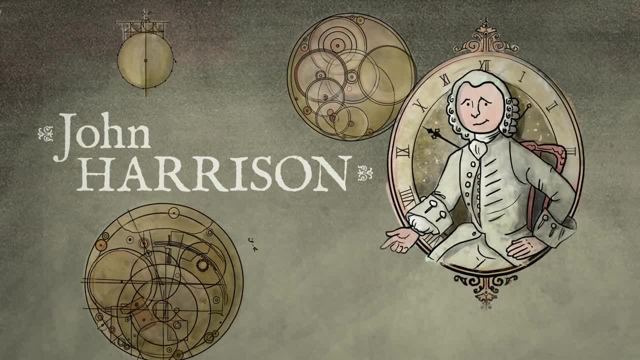 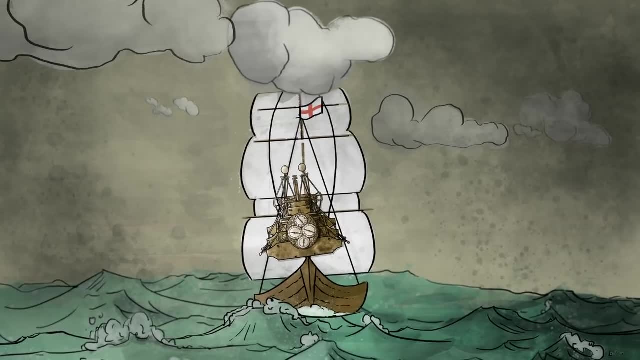 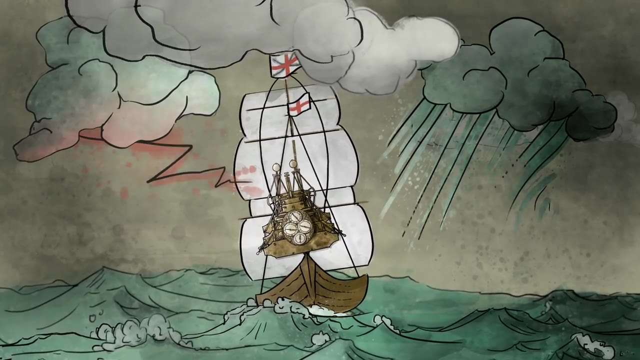 John Harrison, an English clockmaker and carpenter, built a clock that could keep accurate time at sea. A timepiece that could maintain accurate time while on a pitching yawing deck in harsh conditions was necessary in order to know the time back in England. There was one catch, though, Since such 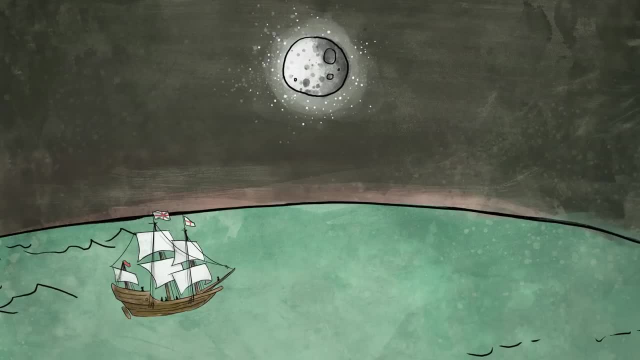 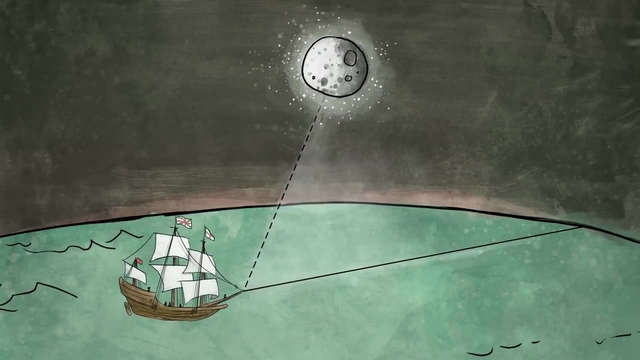 a timepiece was hand-made. the clock could be used to measure the length of the ship. The clock was very expensive, so an alternate method using lunar measurements and intense calculations was often used to cut costs. The calculations to determine a ship's location for each measurement. 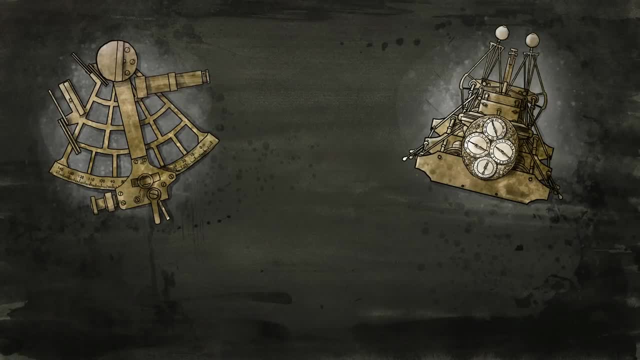 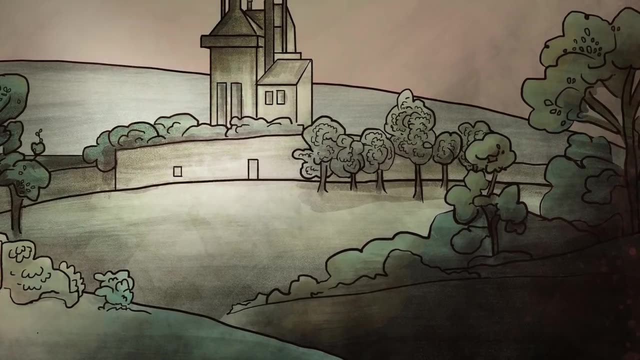 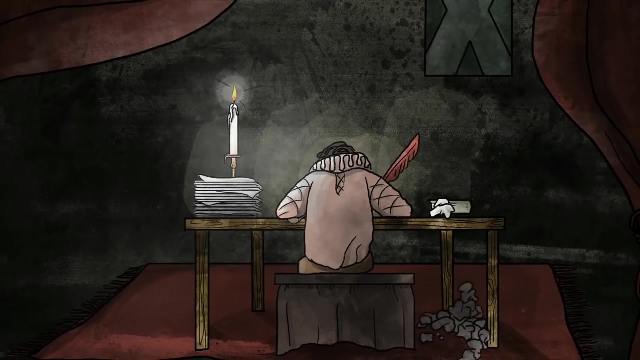 could take hours, But sextants and clocks weren't useful unless sailors could use these tools to determine their position. Fortunately, in the 1600s an amateur mathematician had invented the missing piece. John Napier toiled for more than 20 years to find the missing piece. He 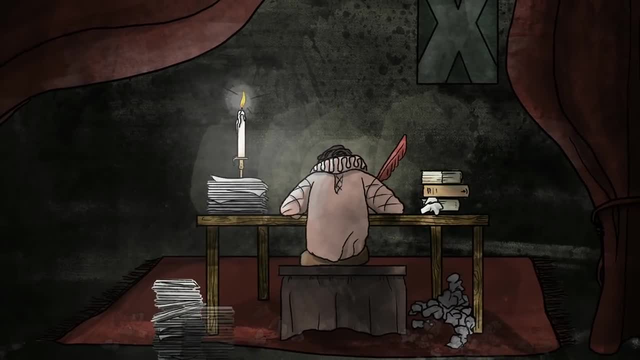 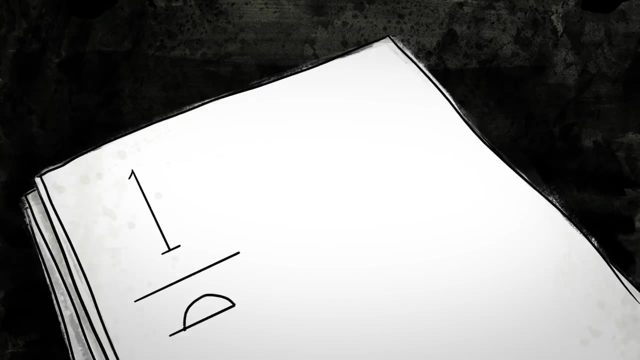 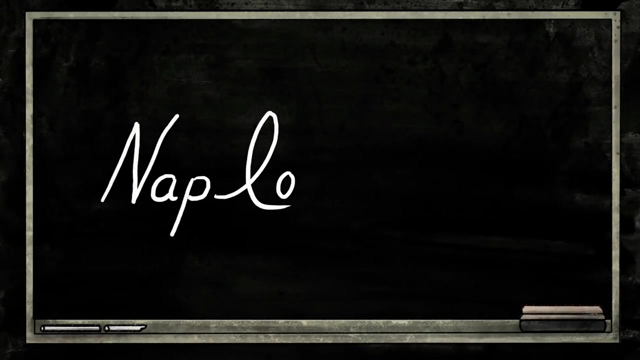 had spent many years in his castle in Scotland to develop logarithms, a calculation device. Napier's ideas on logarithms involved a form of 1 over e and the constant 10 to the seventh power. Algebra in the early 1600s was not fully developed and Napier's logarithm of 1 did not equal zero. 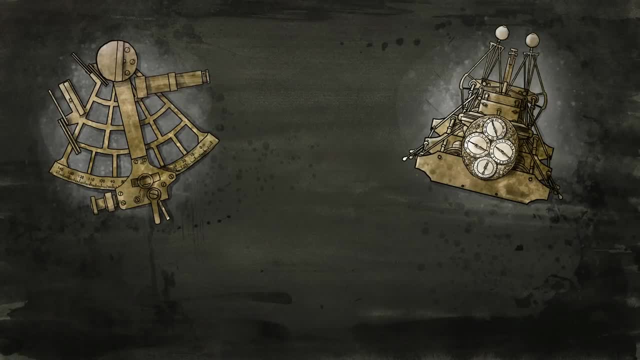 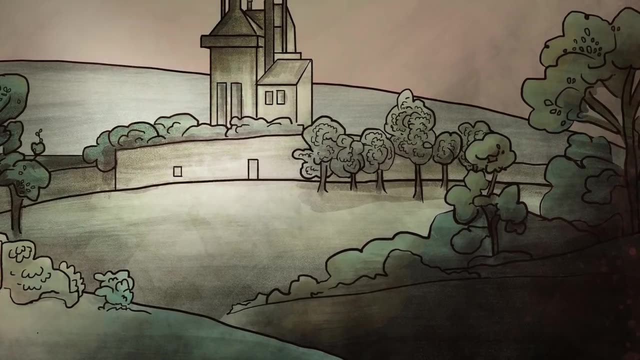 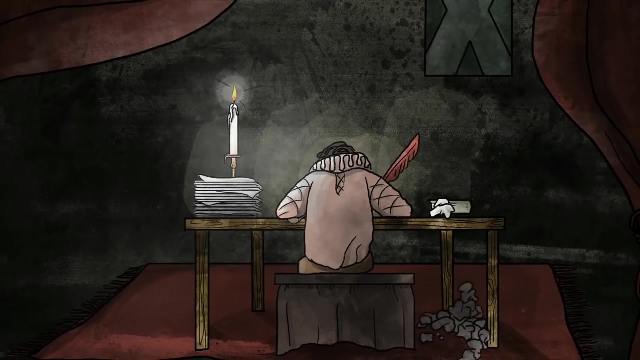 could take hours, But sextants and clocks weren't useful unless sailors could use these tools to determine their position. Fortunately, in the 1600s an amateur mathematician had invented the missing piece. John Napier toiled for more than 20 years to find the missing piece. He 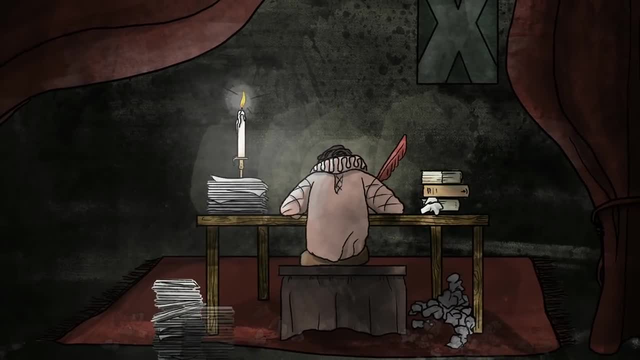 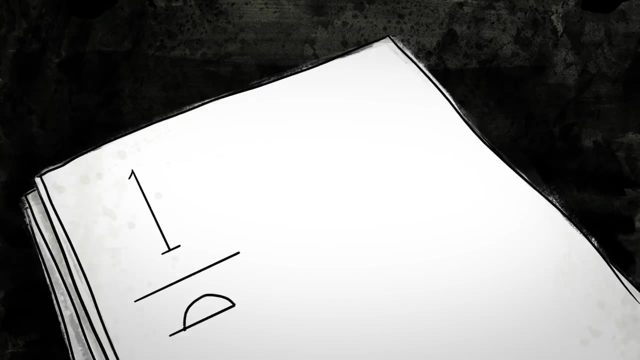 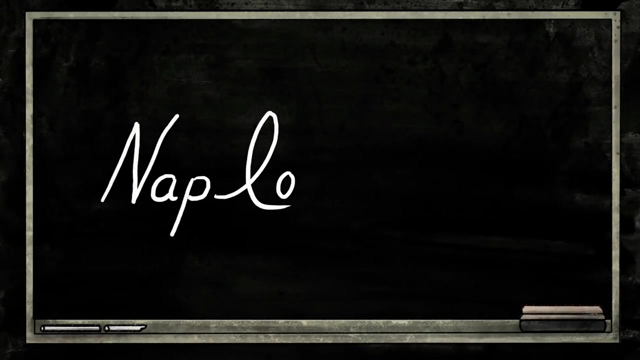 had spent many years in his castle in Scotland to develop logarithms, a calculation device. Napier's ideas on logarithms involved a form of 1 over e and the constant 10 to the seventh power. Algebra in the early 1600s was not fully developed and Napier's logarithm of 1 did not equal zero. 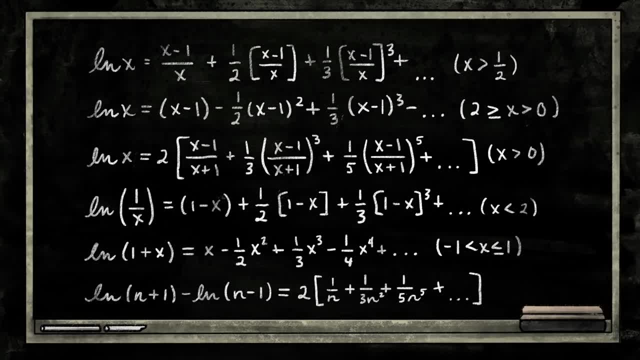 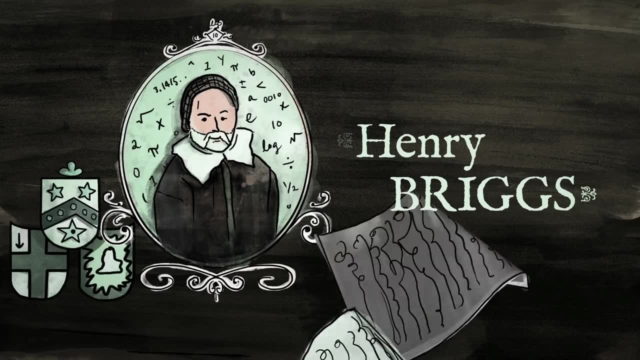 This made the calculations much less convenient than logarithms with a base of 10.. Henry Briggs, a famous mathematician, wrote that the logarithm of 1 was less convenient than the logarithm of 10.. John Napier, a mathematician at Gresham College in London, read Napier's work in 1614 and the 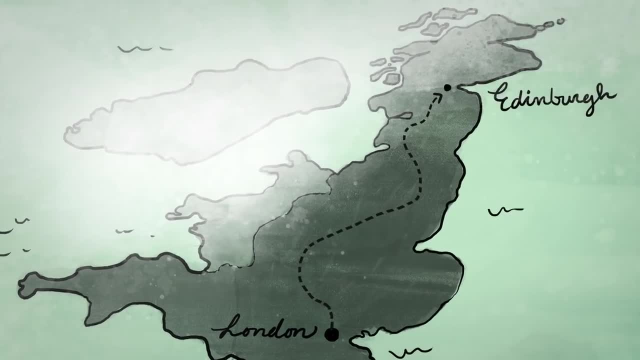 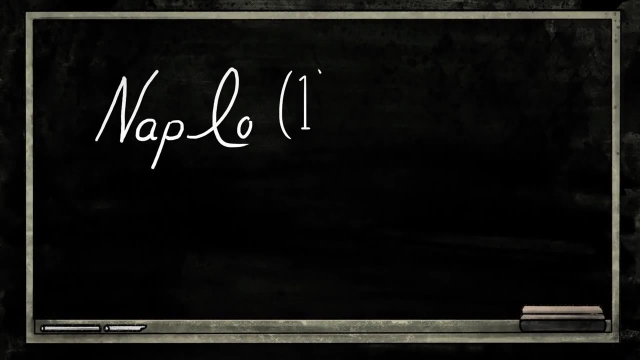 following year made the long journey to Edinburgh to meet Napier. Briggs showed up unannounced at Napier's castle door and suggested that John switch the base and form of his logarithms into something much simpler. They both agreed that a base of 10 with the log of 1 equal to zero would. 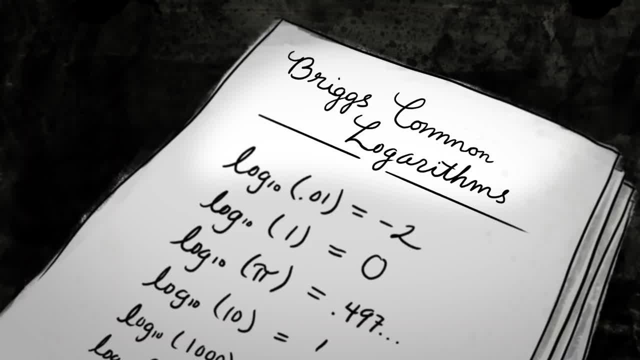 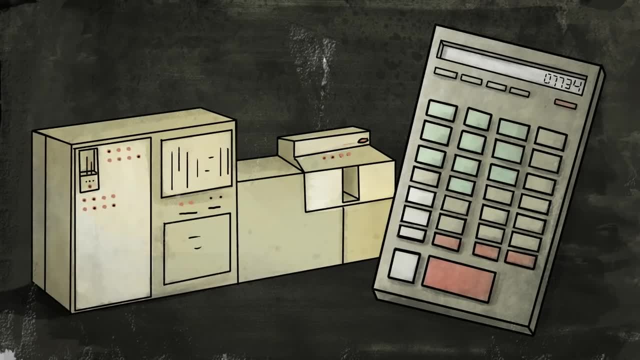 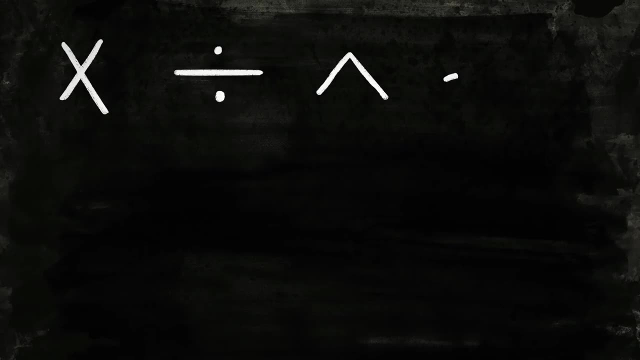 greatly simplify everyday calculations. Today we remember these as Briggs' common logarithms. Until the development of electric calculating machines in the 20th century, any calculations involving multiplication, division powers and extraction of roots with large and small numbers were done using logarithms. 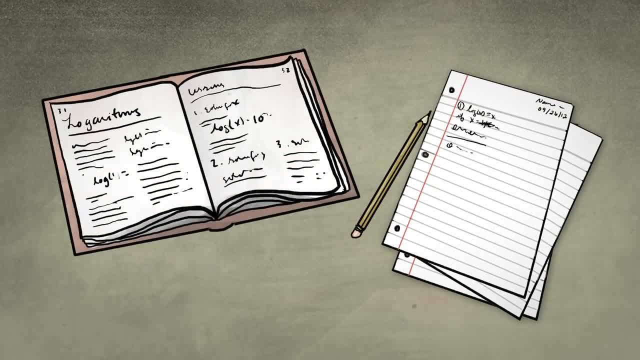 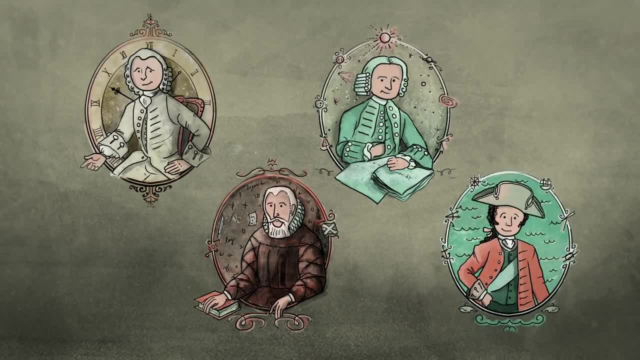 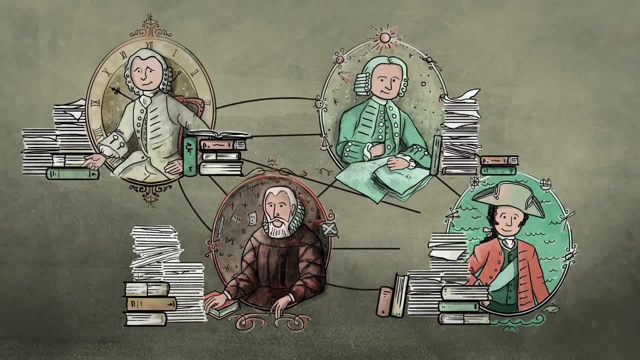 astronomers, mathematicians and, of course, sailors. Creativity isn't only about going deep into one's field of work. it's about cross-pollination between disciplines too.